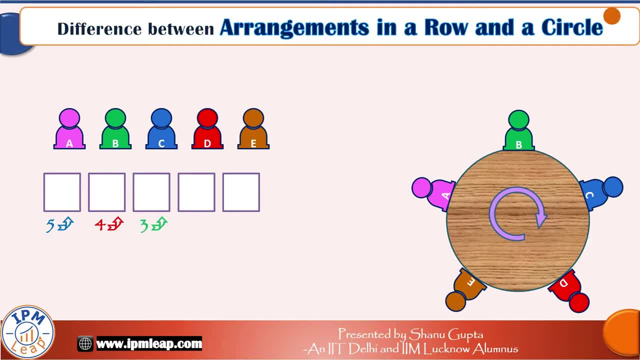 The third slot can then be filled in three ways, The fourth in two ways, And for the last slot we will be left with only one object. So altogether these five objects can be arranged in a row in 5 x 4 x 3 x 2 x 1, ie 5 factorial or 120 ways. 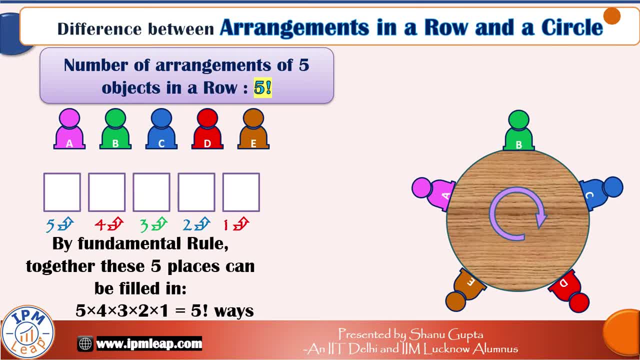 In general, n different objects can be linearly permuted or arranged in n factorial ways. Now, instead of filling the first slot with one object, we can fill the second slot with another object. Now, instead of filling the first slot with one object, we can fill the second slot with another object. 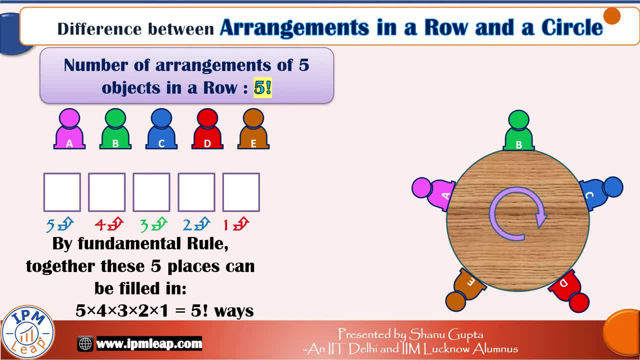 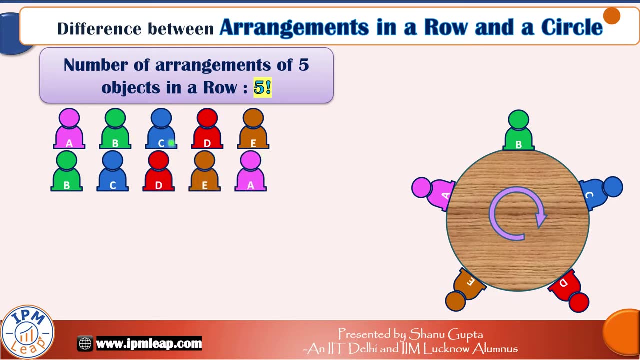 In other words, you could be arranging five persons, but the number of arrangements remain the same: 5 factorial. Please observe these two ways of arranging the five persons. The first one looks like A, B, C, D and E, While in the second one we have shifted all of them. 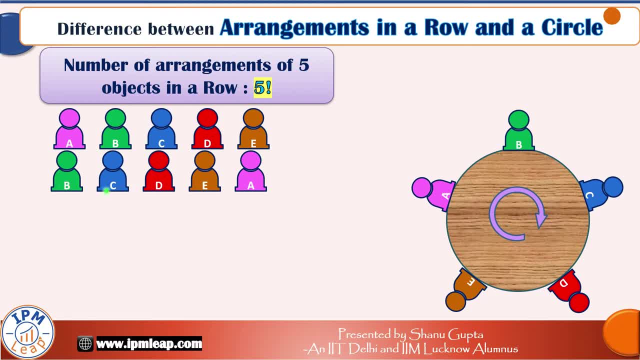 one position to the left and placed A to the extreme right. It looks like B, C, D, E, A. Now the important question is: how do we arrange the five objects? Would you consider these two as same or different? Well, they are obviously different, The very fact that the first arrangement starts with A. 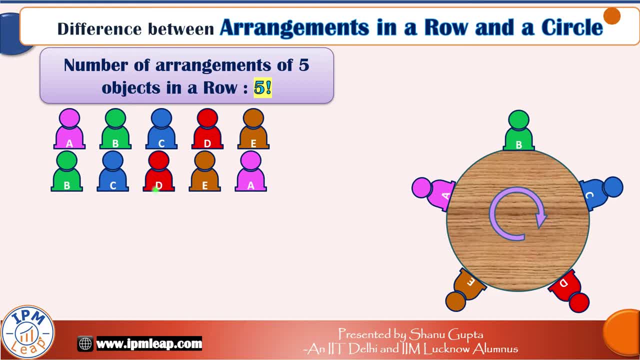 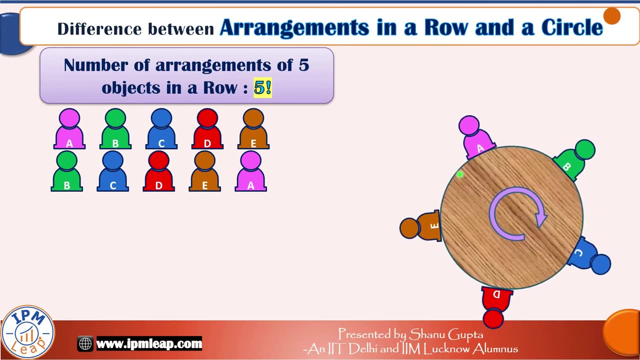 and second starts with B makes them different. Contrast this to a circular arrangement: The same five objects. when arranged around a round table, the configuration looks like this, And if you move along the table in a clockwise direction, you will be able to see both the first and the second arrangement ABCDE, as well as. 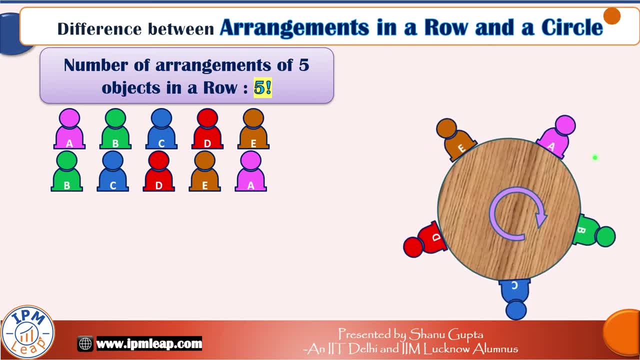 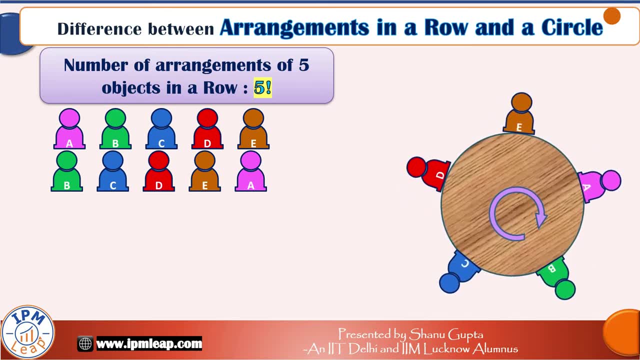 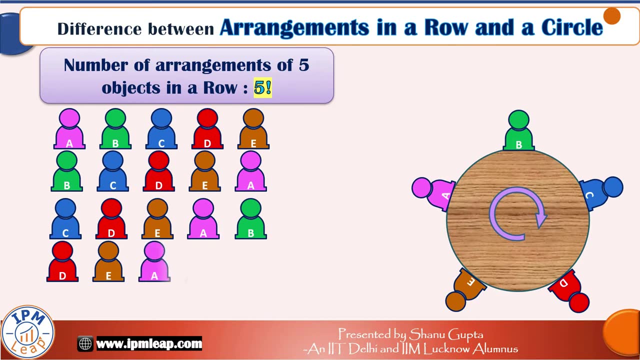 BCDEA in the same configuration of the round table. In fact, if you start at C, you will additionally observe the arrangement C, DEA B, If you start at D, you will observe the arrangement DEABC, and if you start at E, you will. 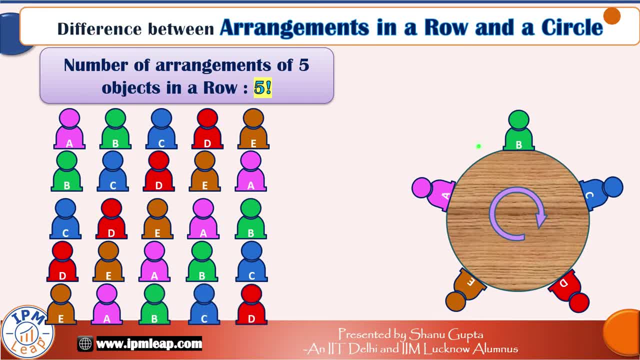 be able to observe EDEAB. In a row arrangement, we need to take into consideration the position of all the persons or objects, But at the round table it all depends on where you start. it's all relative. This is because a circle has no starting or ending point. 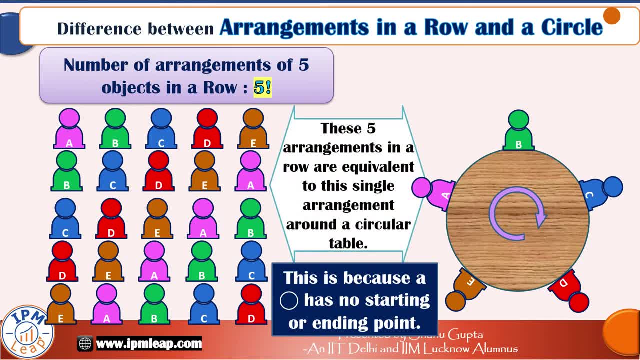 So these five arrangements, which are counted as different in linear arrangements, become the same in a circular arrangement. In both cases, a, b, c, d, e have been arranged in a clockwise order, isn't it? So can I say that these five arrangements in a row are equivalent to this single arrangement? 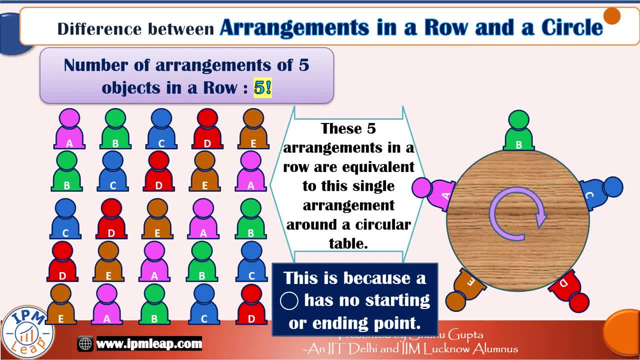 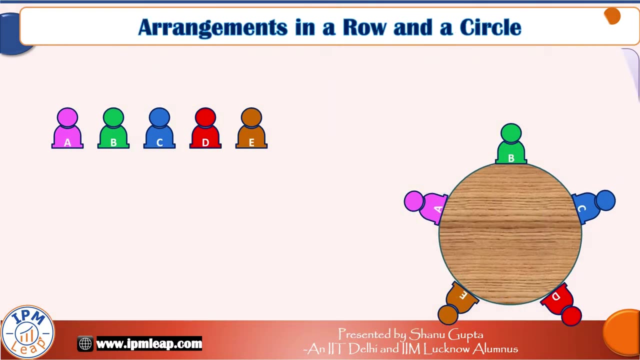 around a circular table. Yes, of course, And therefore for counting the number of circular arrangements in this example, we must divide the number of linear arrangements by 5.. 5 factorial divided by 5 is 4 factorial. Ok, That's why the number of arrangements of 5 objects around the circle is 4 factorial. 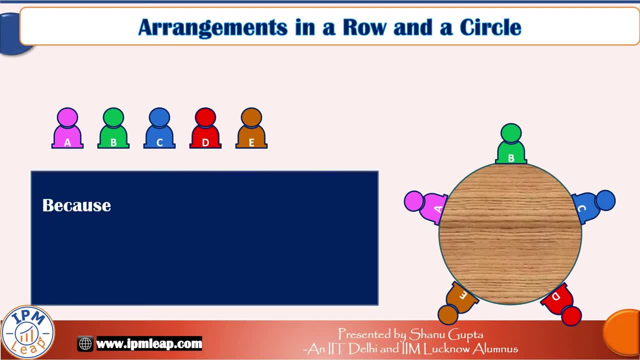 Now that you have understood that in a circle which has no starting or ending point, we observe arrangements related to any one of the objects, there is a very simple approach that will help us solve all questions on circular permutation, without exception. What we must do is we fix any problem. 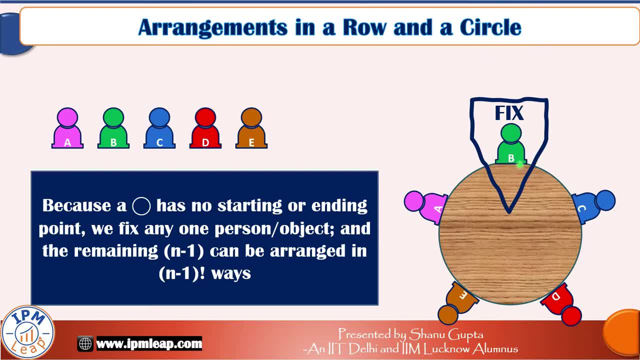 Any one of them say: you can fix b or even c or even a, And next we see how many arrangements of the remaining n-1 objects are possible with respect to that fixed object. The remaining n-1 objects can be arranged in n-1 positions in n-1 factorial ways. 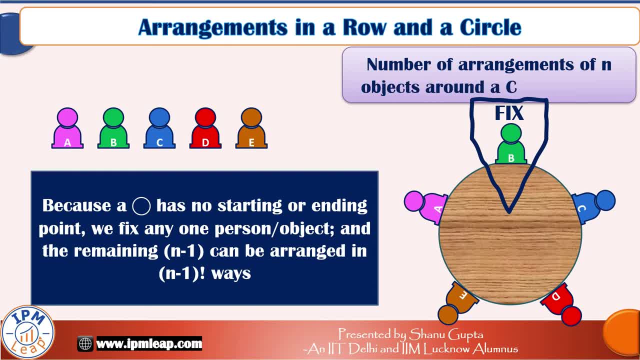 Therefore, the number of ways of arranging n objects around a circular table is 4 factorial. So the number of ways of arranging n objects around a circular table is n-1 factorial. On the other hand, when we have a row or straight line, there are n factorial ways of arranging. 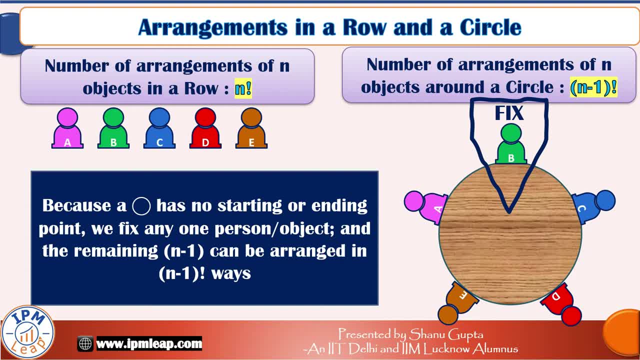 n persons or n distinct objects. So 5 people can be arranged around a circular table in 5-1 factorial, ie 4 factorial or 24 ways. Let's try to attempt a few questions on circular permutations where there are n-1 objects. 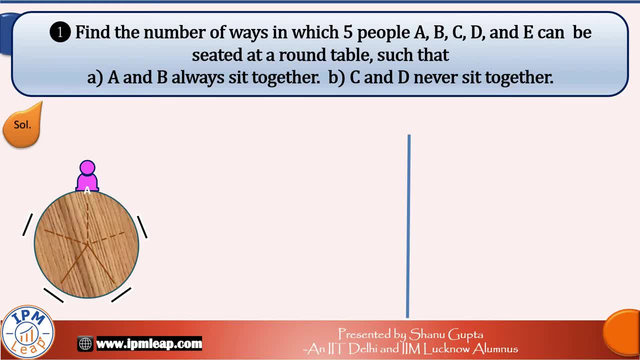 So let's try to attempt a few questions on circular permutations, where there are n-1 objects and there are other restrictions as well. So find the number of ways in which 5 people- a, b, c, d, e- can be seated at a round table. 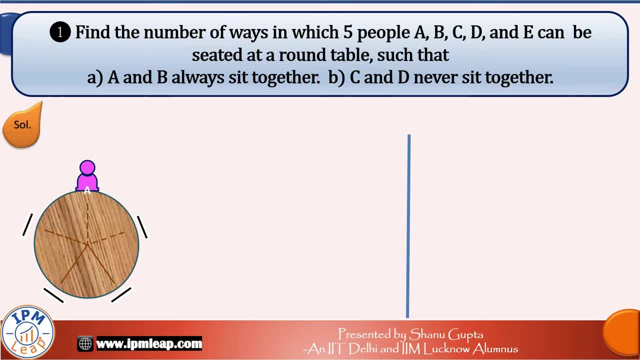 such that a and b always sit together. We have learnt that five people can be arranged on a round table in 4 factorial. that is 24 ways. Always remember, guys, Any circular permutation question. first we choose the particular person that we need to fix. 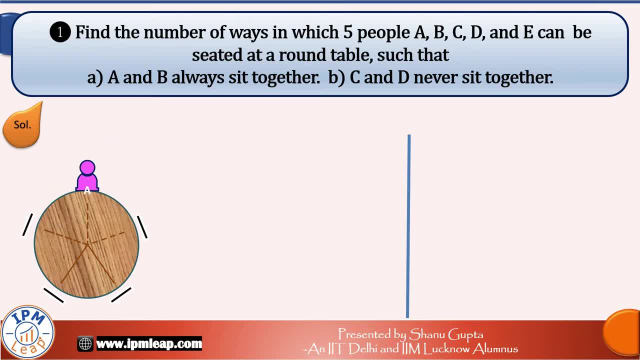 and after that we address other restrictions. So in this question, if A and B must sit together, let's fix A. That will make our question simpler. A got seated in one way. Now B sits either to his left or to his right. Therefore B can be seated in two ways. Once we have seated B, say on the left. 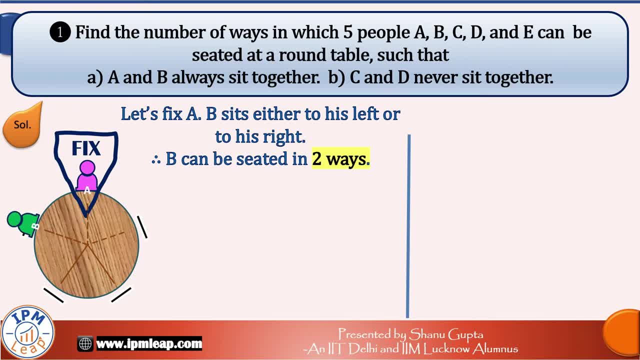 there are no more restrictions. So the remaining three people can be seated in the remaining three seats in three factorial. that is six ways. Recall that n people can be arranged in n positions in n factorial ways. By using the fundamental rule of counting together, we can get the following rules: 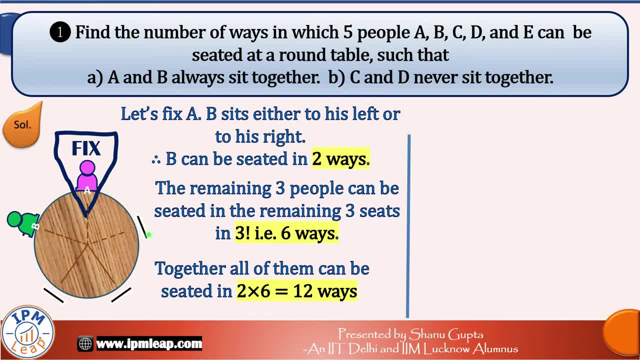 A and B, and then the rest of the persons can be seated in 2 into 6, that is 12 ways. Part B of this question is: C and D never sit together, which means C and D are separated. We can follow a very simple approach here. Number of ways where C and D are separated. 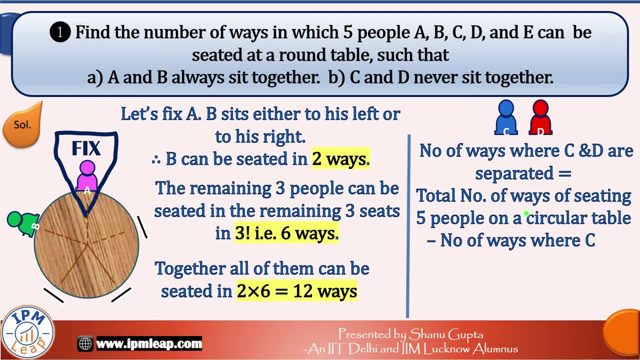 is equal to total number of ways of seating five people on a circular table, which is 4 factorial minus the number of ways where C and D are together. Now it's obvious from part A of this question that if A and B were seated together in 12 ways, then C and D or for. 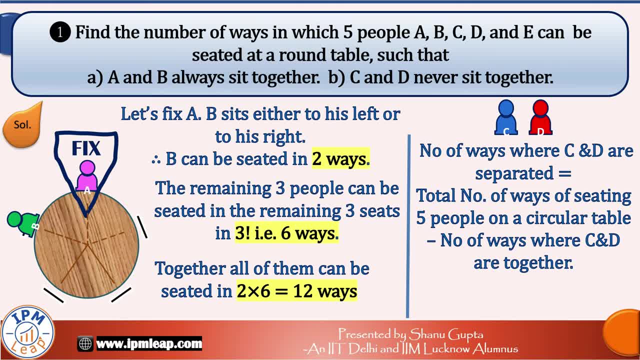 that matter, any other pair would also be together in exactly 12 ways. So our answer is 4 factorial minus 12, which is equal to 12 ways. Another approach for the same question is to see the number of ways where C and D are separated. 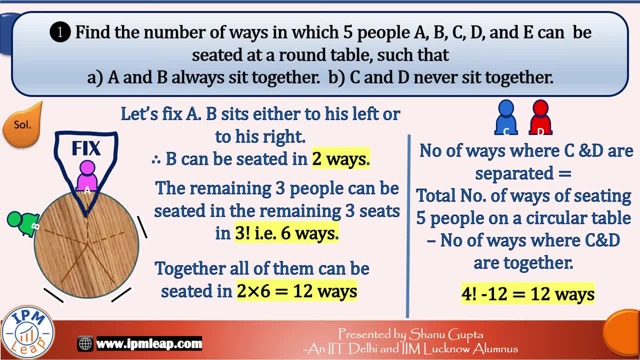 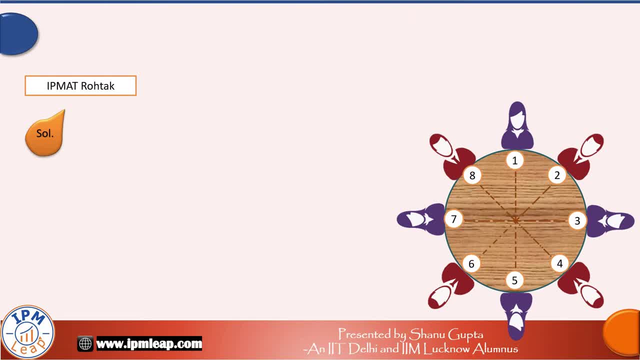 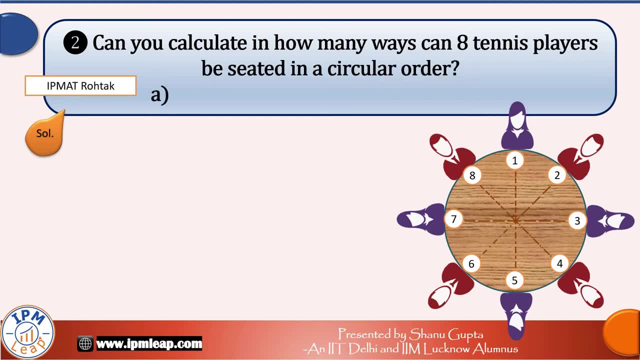 Another approach for the same question is illustrated in question number 3 of this video. Next question is quite straightforward. It was asked in IPMAT IIM Rohtak: Can you calculate in how many ways 8 tennis players be seated in a circular order? 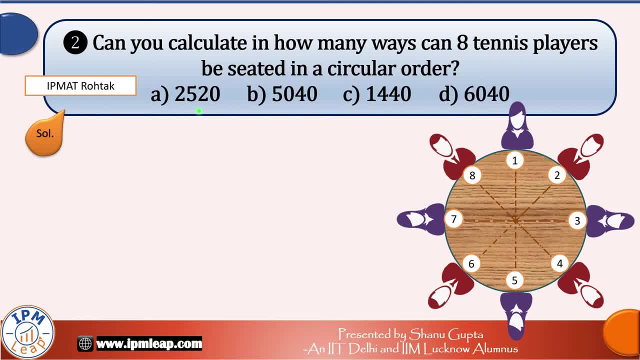 And the options are 2520,, 5040,, 1440 and 6040.. Now we know that n people can be arranged around a circular table in n-1 factorial ways. Therefore, 8 tennis players can be arranged around a circular table in 8-1 factorial, ie 7 factorial ways. 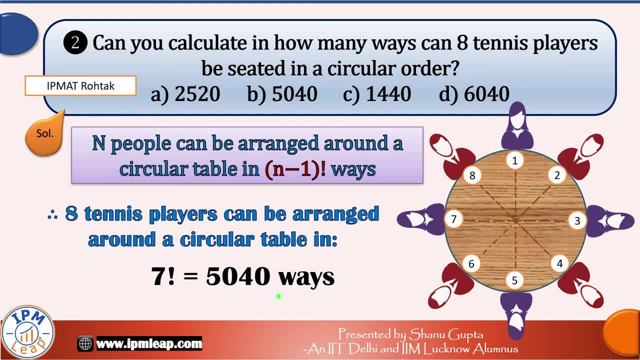 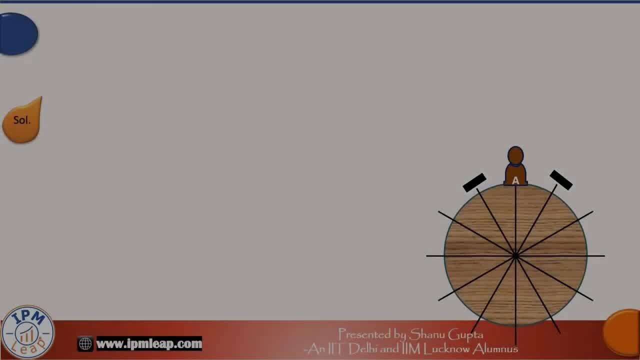 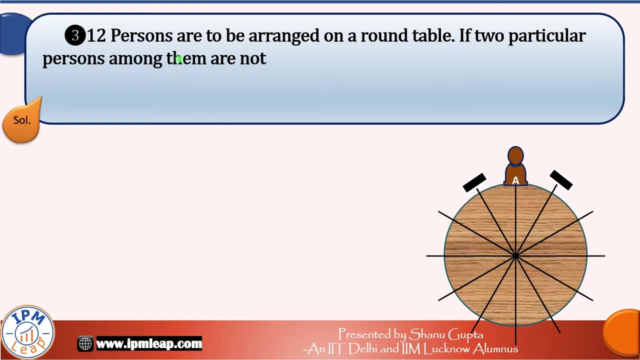 7 factorial evaluates to 5040.. That's it. Option B is our correct answer. Third question is: 12 persons are to be arranged on a round table If two particular persons among them are not to be seated side by side. 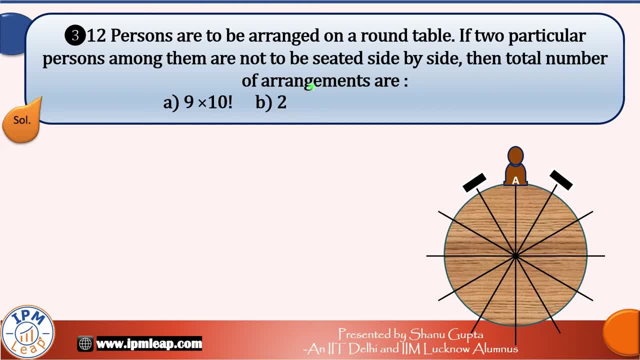 then total number of arrangements are And we have to choose one of the options. So don't forget any circular permutation question. look at the restrictions and address them first. You will also get a clue about the person to be fixed, seeing those restrictions. 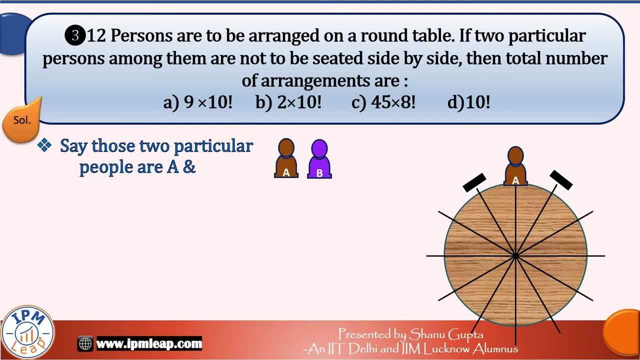 So let's say those two particular people are A and B. Let's fix A. Next, we must ensure that B does not sit on either of the seats adjacent to A, because that's the only restriction in the arrangement of these people. So let's fill the adjacent seats to the left and right of A. 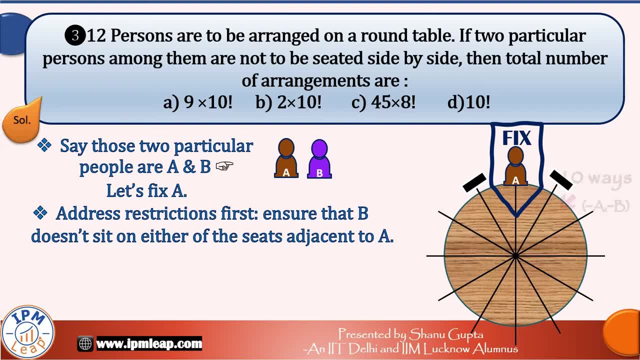 the person we have fixed before we fill the remaining seats. So this seat we can't fill A because A is already seated and we can't fill B. How many left? 12-2, ie 10 people. This seat can be filled in 10 ways. 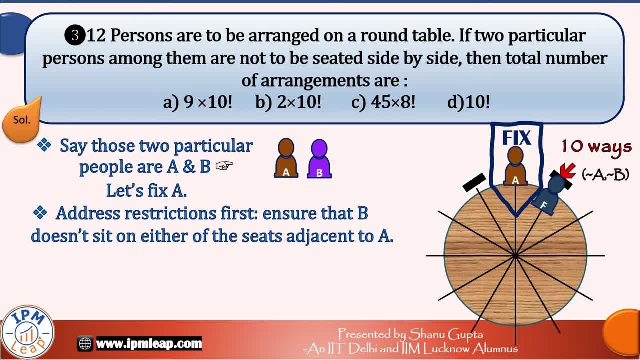 And any other person except B, say F, gets seated here Next we fill this seat. We can't fill A and F because they are already seated on the round table And we can't fill B. How many left? 12-3, ie 9 persons. 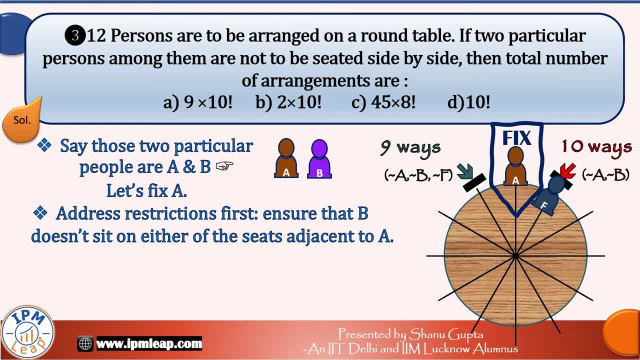 This seat can be filled in 9 ways. Now we don't have any other restrictions, So the remaining 9 seats can be filled with remaining 9 people, including B, in 9 factorial ways. Therefore, all 12 people can be seated in 10 x 9 x 9 factorial. 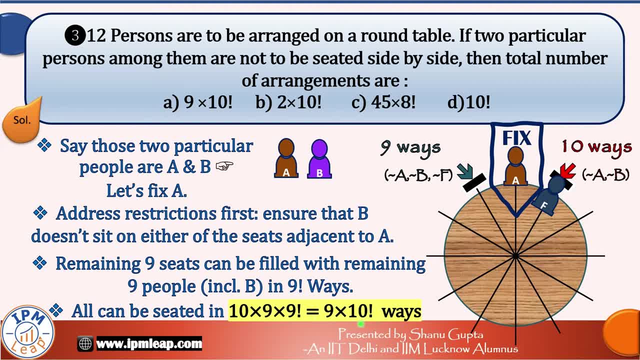 which is equal to 9 x 10 factorial ways. I have used the fundamental rule of counting here. You may watch our other lessons on permutations and combinations, including the fundamental rule, if you feel you need to revise them. Our answer for this question is option A. 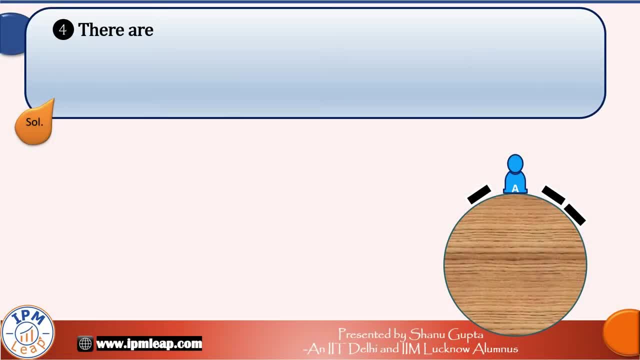 Fourth question is: There are two brothers among a group of 20 persons. In how many ways can the group be arranged around a circular table so that there is exactly one person between the two brothers? And these are the options. So suppose that those brothers are A and A'. 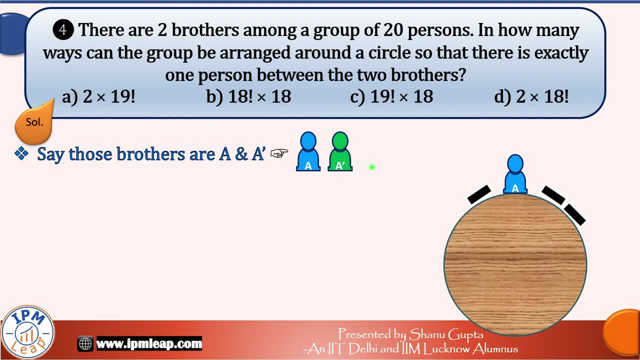 First we will fix one of them, say the blue one, A. Now A' sits either to the left or to the right, leaving a gap of one seat in both cases, isn't it? That means A' can be seated in two ways. 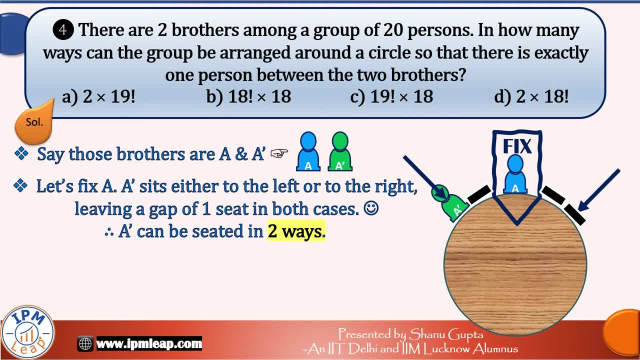 We don't have any more restrictions now. Out of the 20 persons- A and A', two of them are already seated And the remaining 18 seats can be filled with the remaining 18 people in 18 factorial ways. So by using the fundamental rule of counting, 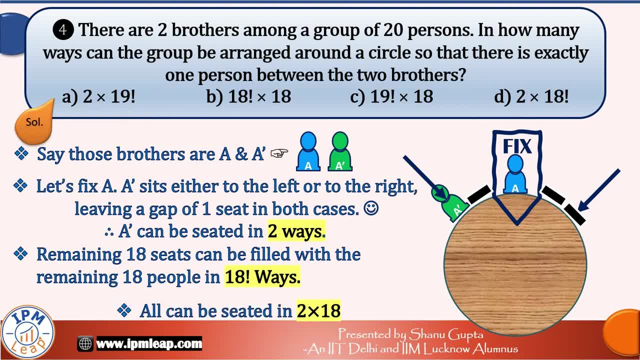 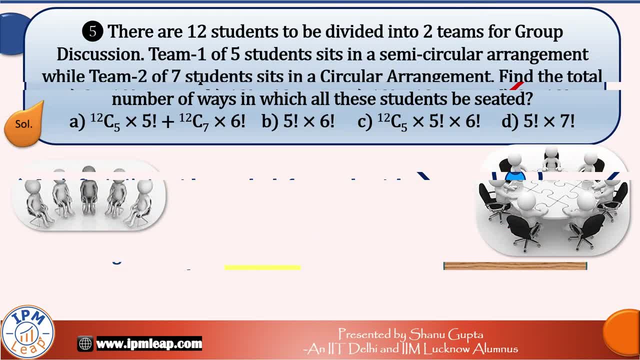 all 20 persons can be seated in 2 x 18 factorial ways. So option D is our correct answer And this one is my favourite. I have taught this as an example to most people. I have given an example to multiple batches of students. 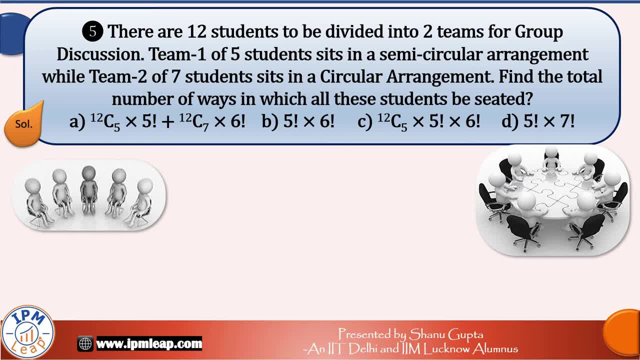 for over 10 years. The question is: there are 12 students to be divided into two teams for group discussions. Team number 1 of 5 students sits in a semi-circular arrangement, while team number 2 of 7 students sits in a circular arrangement. 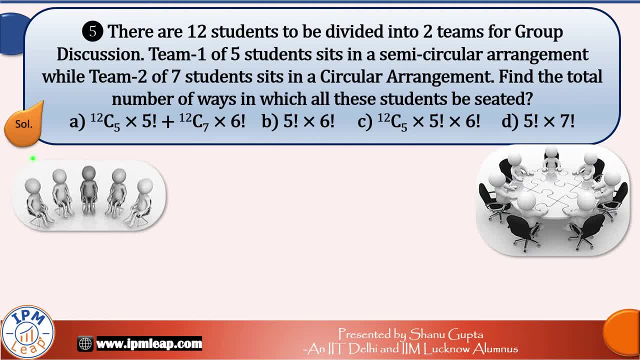 Find the total number of ways in which all these students be seated? This is a classic question combining the basics of combinations, linear permutations and circular permutations, And the options are really tricky. So listen carefully. If we knew which 5 students would go into team 1,. 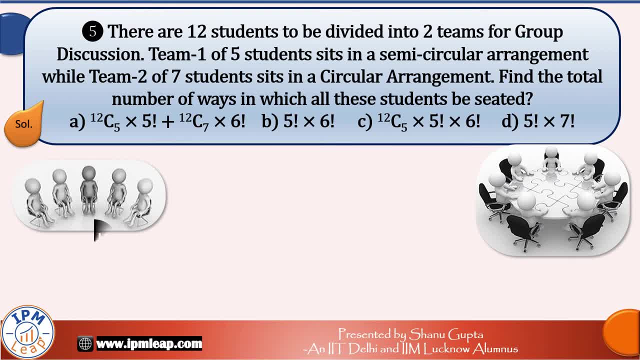 they would be seated in 5 factorial ways, Because that's very much like a linear arrangement. It has a start and an end. Similarly, if we knew which 7 students will go into team 2, they could be seated in 6 factorial ways. 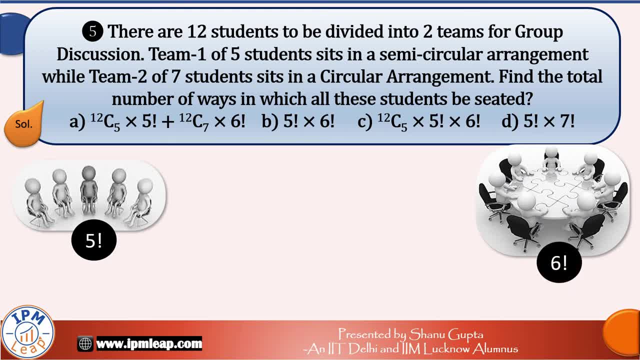 But in the beginning we don't know who goes where. So first the GD committee selects students for both teams. That can be done in 12C5 ways. The moment 5 students get shortlisted for team 1, obviously the remaining 7 go to team 2.. 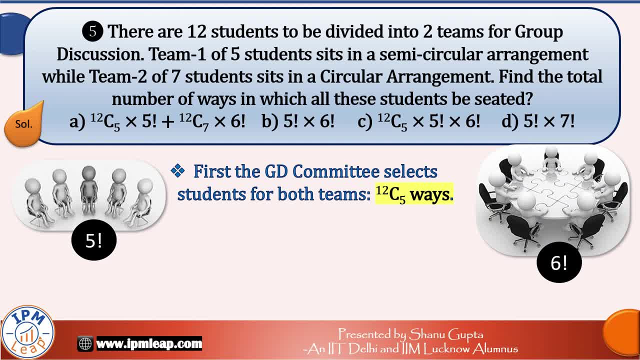 So for team 2, we don't need a fresh selection. In any case, recall that 12C5 is equal to 12C7.. This selection needs to be done only and only once. Then comes the arrangement part, Once selected. 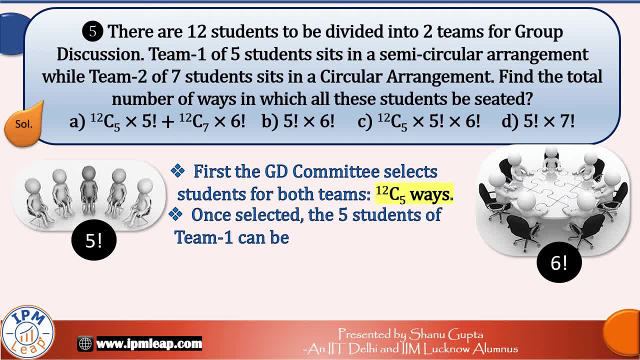 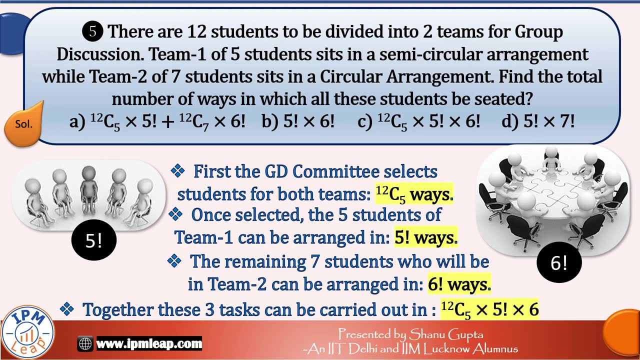 the 5 students of team 1 can be arranged in 5 factorial ways. The remaining 7 students who will be in team 2 can be arranged in 6 factorial ways. Together, the 3 tasks above can be carried out in 12C5 into 5 factorial, into 6 factorial ways. 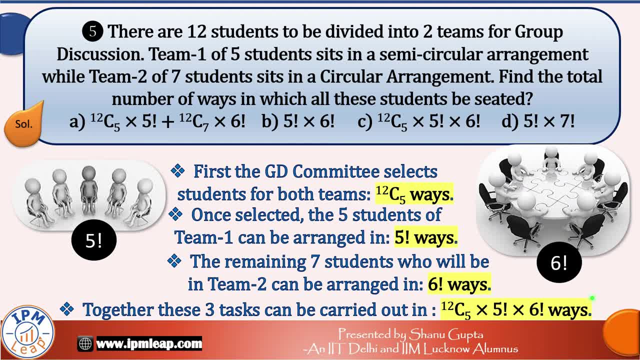 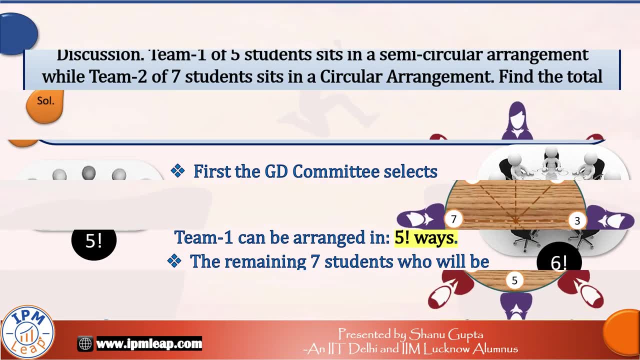 using the fundamental rule of counting, Because we need to select students for both teams and arrange team 1 and arrange team 2, we need to multiply And means multiply Okay. So option C is our correct answer. Finally, we have the question. 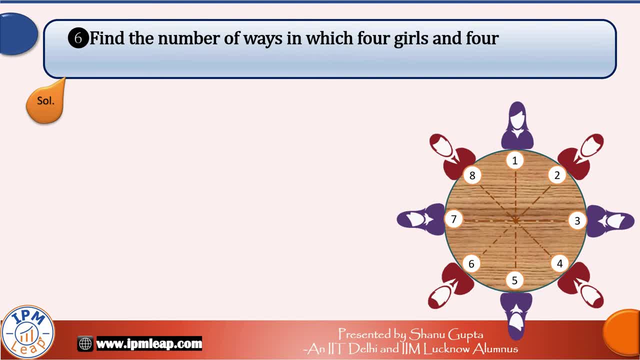 find the number of ways in which 4 girls and 4 boys can be arranged around a circular table so that none of the boys are together. For this condition to be met- that boys are separated- girls and boys must be seated alternately. 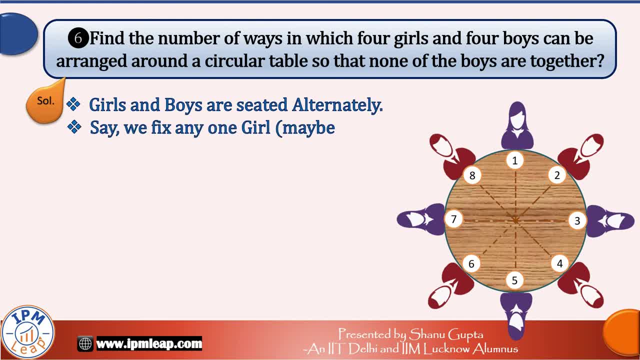 So suppose we fix, any one girl may be G3, on position number 1.. That can be done in only one way. Position number 3, number 5, number 7 can be occupied by the remaining 3 girls in 3 factorial ways. 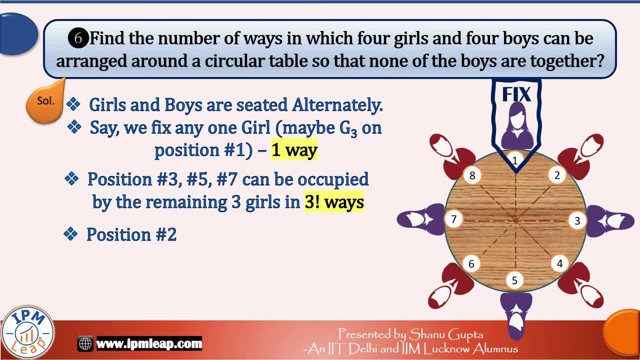 And position number 2, number 4, number 6 and number 8 can be occupied by the 4 boys in 4 factorial ways Together. all girls and boys, remember that. and means multiply. They can be seated in 3 factorial into 4 factorial ways. 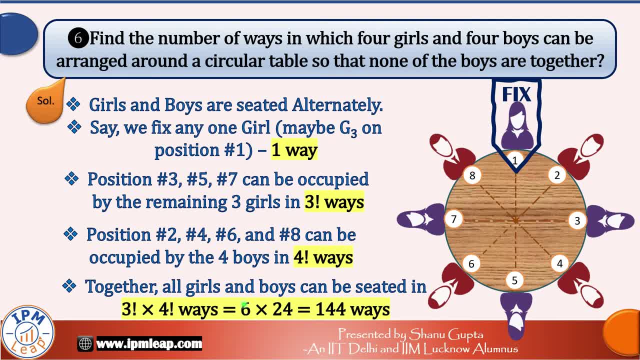 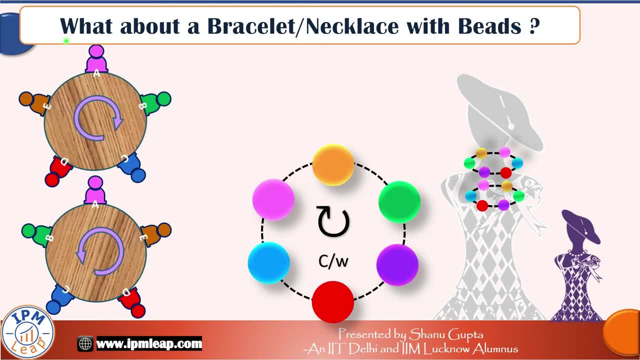 which is equal to 6 into 24, that is 144 ways. Now we come to a very special instance of circular permutation, where we have a bracelet or necklace with multicolored beads. In how many ways can you string together 6 beads? 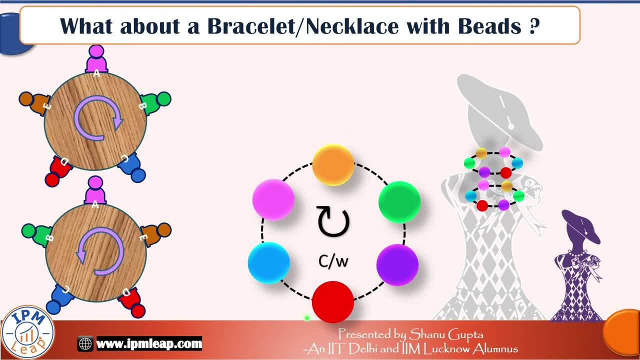 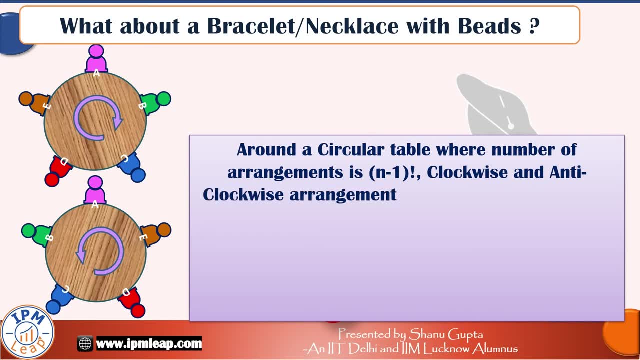 to form a necklace. So we have already studied that around a circular table the number of arrangements is n-1- factorial. In this n-1 factorial ways, clockwise and anticlockwise arrangement of objects are counted as different. This is because a table cannot be flipped. 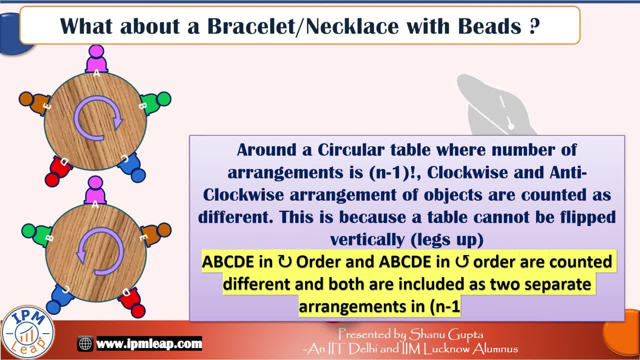 vertically. legs are Okay. so ABCDE in clockwise order and ABCDE in anticlockwise order are considered different and both are included as two separate arrangements in n-1 factorial ways. But the same is not true for a necklace. Consider the following arrangement: 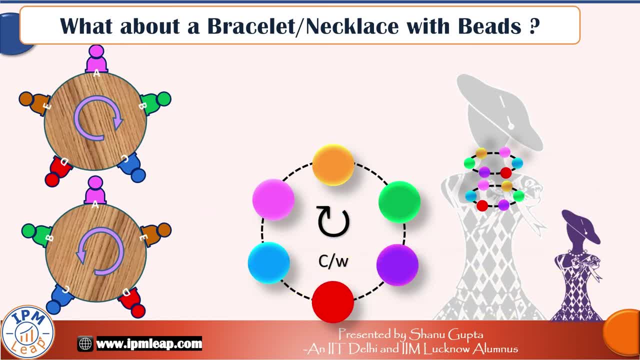 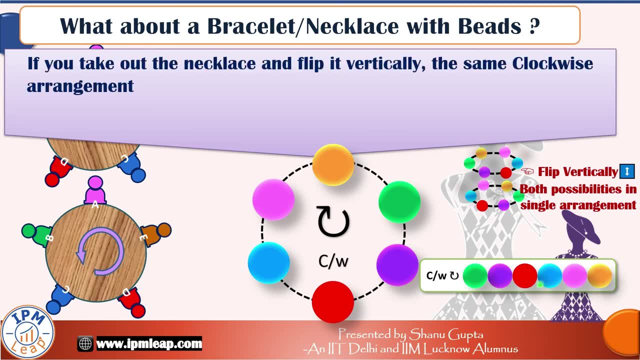 of beads in a clockwise order: Green, purple, red, blue, pink and yellow. If you take out the necklace and flip it vertically, the same clockwise arrangement of beads becomes anticlockwise, Isn't it? Let me show this flip animation. 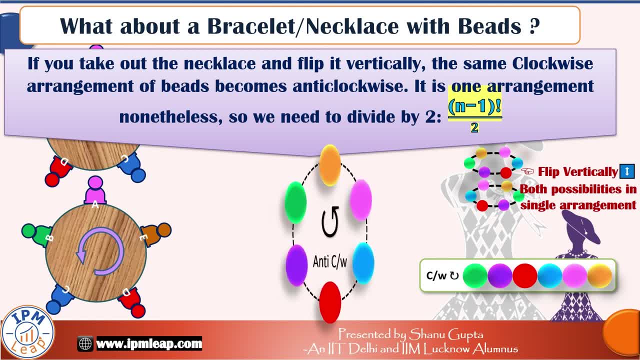 so that you can visualize this happening, See again. And obviously we have not reassembled the beads on the necklace. It's the same arrangement of beads. Clockwise and anticlockwise are not considered different. So we need to divide our number of circular permutations. 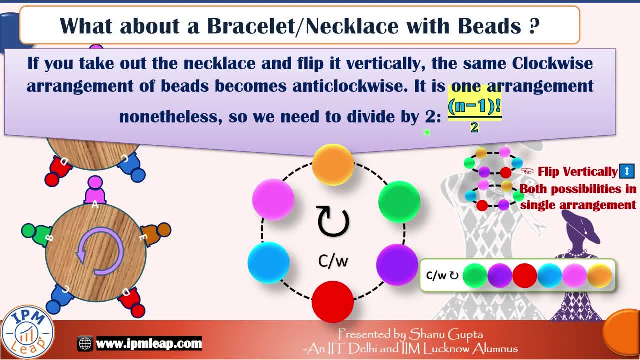 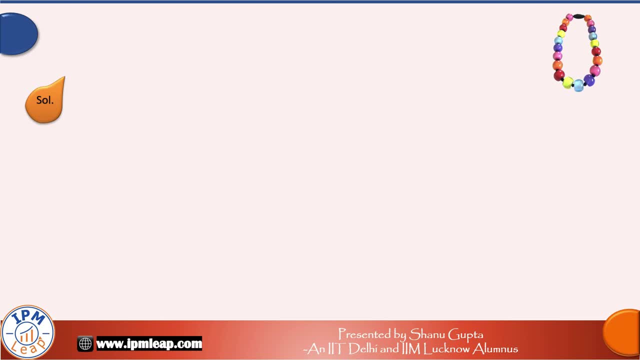 by 2 to account for this. n-1 factorial by 2.. N different beads can be arranged in circular necklace in n-1 factorial divided by 2 ways. So in this last question on circular permutations we have to apply this simple concept.